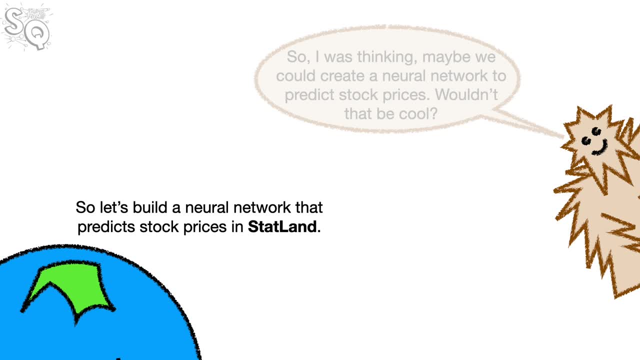 there are far fewer lawyers, So let's build a neural network that predicts stock prices in StatLand. However, first let's just talk about stock market data in general. When we look at stock prices, they tend to change over time. 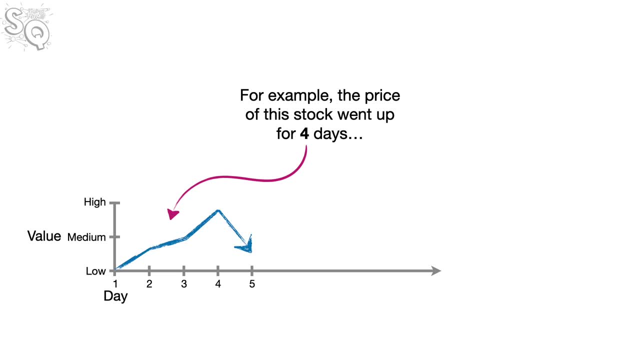 For example, the price of this stock went up for four days- Hooray- Before going down, Wah, wah. Also, the longer a company has been traded on the stock market, the more data will have for it. For example, we have more time points for the company represented by the blue line. 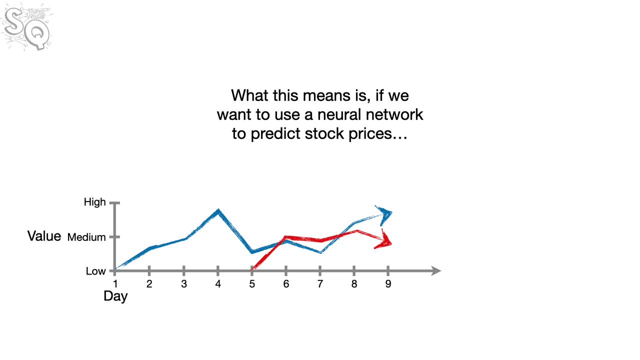 we have for the company represented by the red line. What that means is, if we want to use a neural network to predict stock prices, then we need a neural network that works with different amounts of sequential data. In other words, if we want to predict the stock price for the blue line, 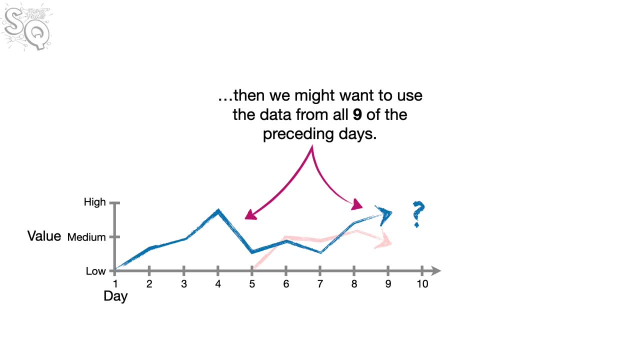 company on day 10,, then we might want to use the data from all nine of the preceding days. In contrast, if we wanted to predict the stock price for the red line company on day 10,, then we would only have data for the preceding five days. So we need the neural network to 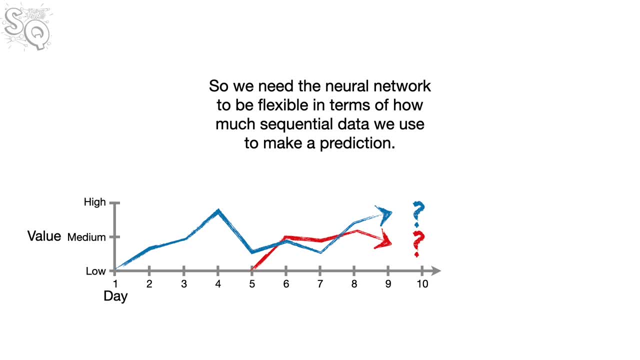 be flexible in terms of how much sequential data we use to make a prediction. This is a big difference compared to the other neural networks we've looked at in this series. For example, in Neural Networks Clearly Explained, we examined a neural network that made predictions. 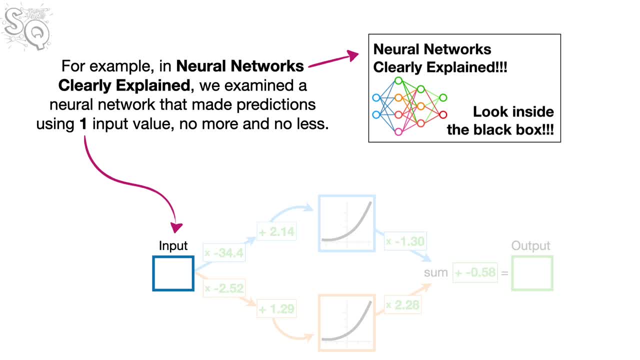 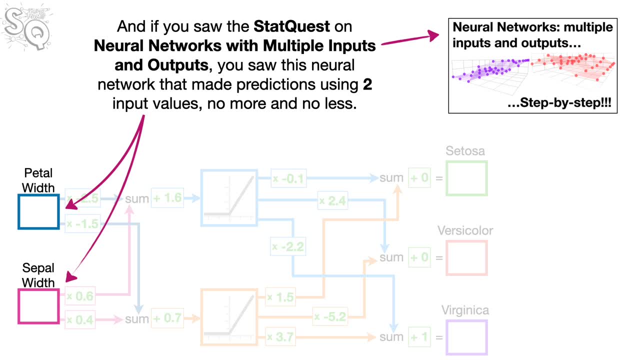 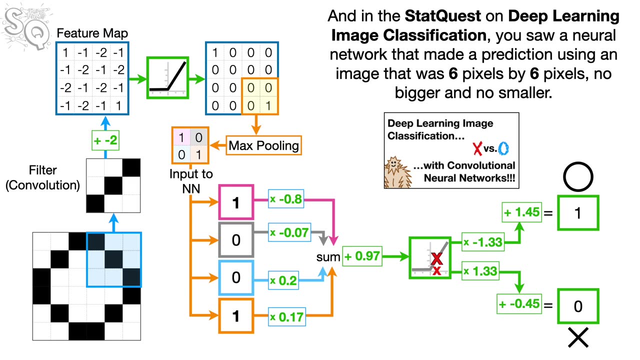 using one input value, no more and no less. And if you saw the StatQuest on neural networks with multiple inputs and outputs, you saw this neural network that made predictions using two input values, no more and no less. And in the StatQuest on Deep Learning Image Classification, you saw a. 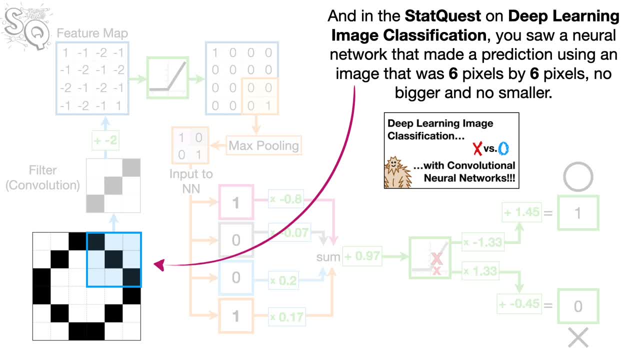 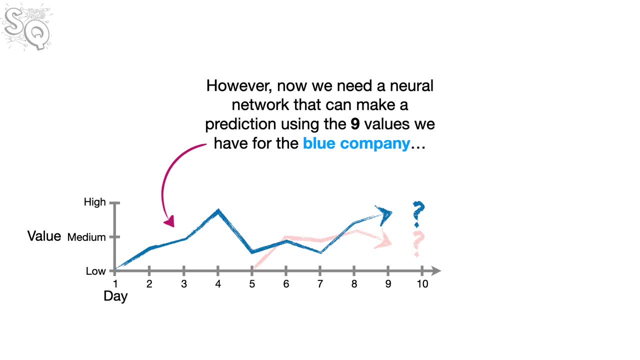 neural network that made a prediction using an image that was six pixels by six pixels, no bigger and no smaller. However, now we're going to look at a neural network that made a prediction using the nine values we have for the blue company and make a prediction using the five. 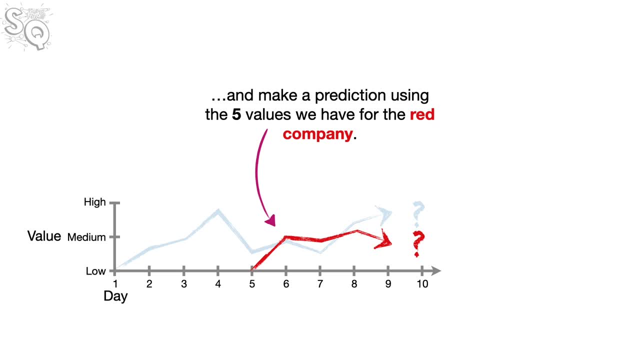 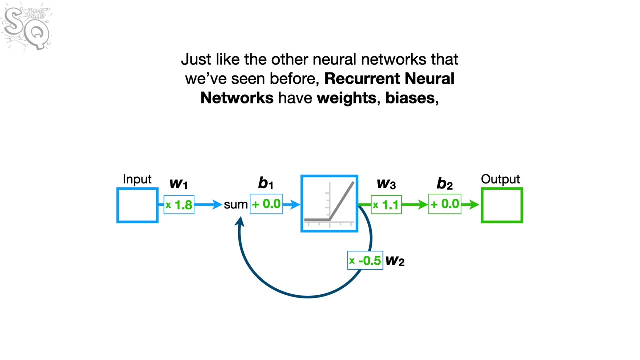 values we have for the red company. The good news is that one way to deal with the problem of having different amounts of input values is to use a Recurrent Neural Network. Just like the other neural networks that we've seen before, Recurrent Neural Networks have weights, biases. 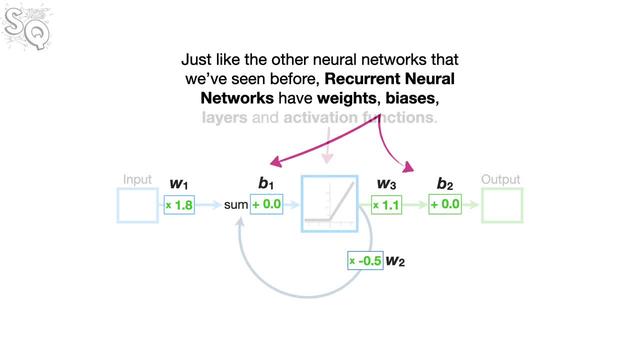 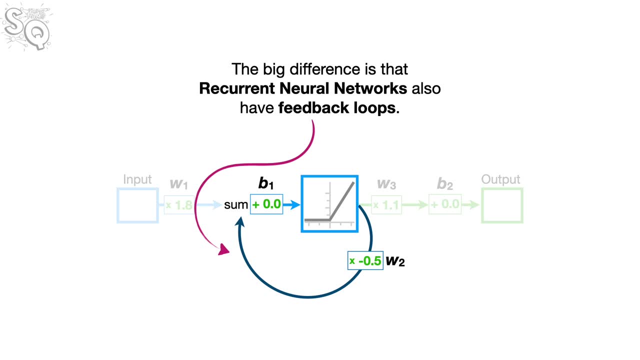 layers and activation functions In the StatQuest on Deep Learning Image Classification. the big difference is that Recurrent Neural Networks also have feedback loops And, although this neural network may look like it only takes a single input value, the feedback loop makes it possible to use sequential input values. 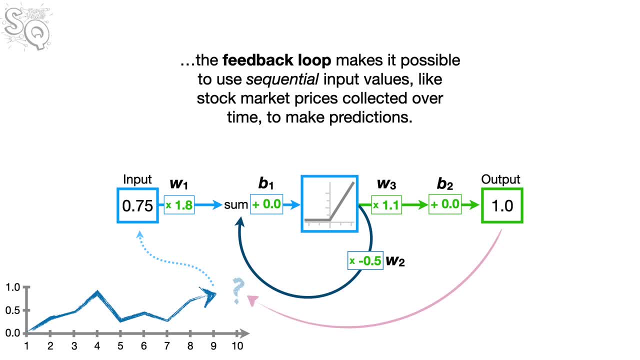 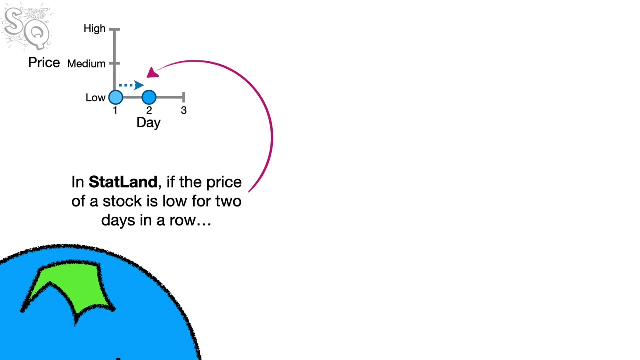 like stock market prices collected over time, to make predictions. To understand how exactly this Recurrent Neural Network can make predictions with sequential input values, let's run some of the stock market data through it In StatLand, if the price of a stock is low for two days in a row, 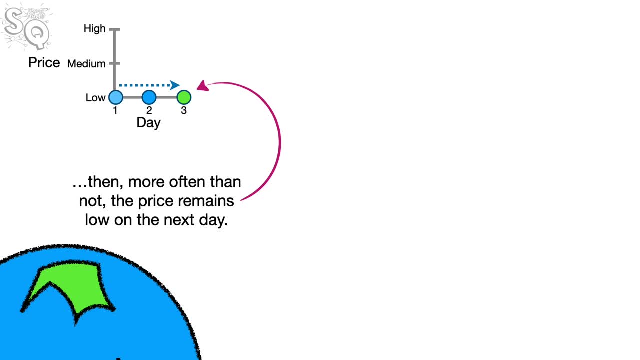 then more often than not, the price remains low on the next day. In other words, if yesterday and today's stock price is low, then tomorrow's price should also be low. In contrast, if yesterday's price was low and today's price is medium, then tomorrow's price should be even higher. 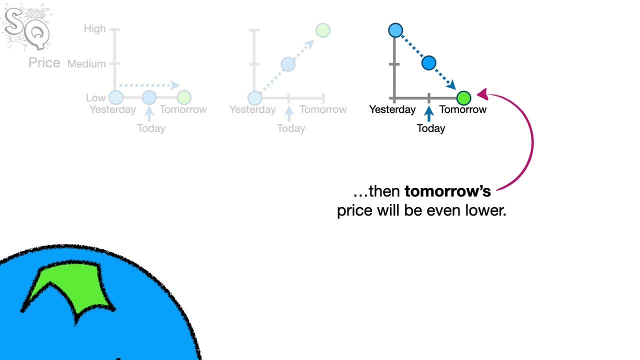 When the price decreases from high to medium, then tomorrow's price will be even lower. Lastly, if the price stays high for two days in a row, then the price will be high tomorrow, Now that we see the general trends in stock prices in StatLand. 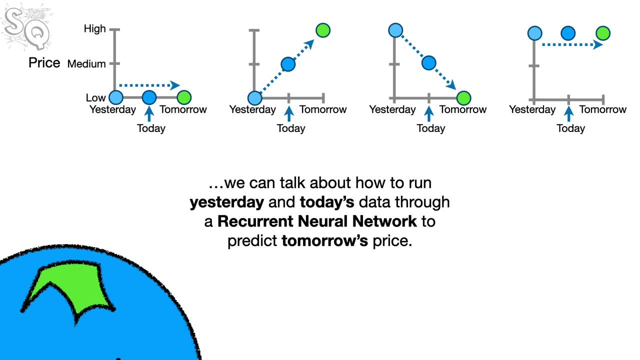 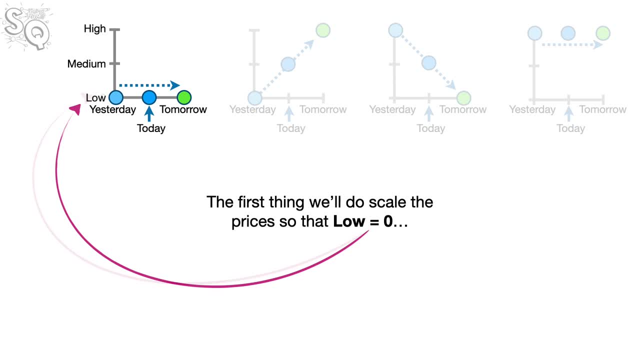 we can talk about how to run yesterday and today's data through a Recurrent Neural Network to predict tomorrow's price. The first thing we'll do is scale the prices so that low equals zero, Medium equals 0.5 and high equals 1.. Now let's run the values for yesterday and today. 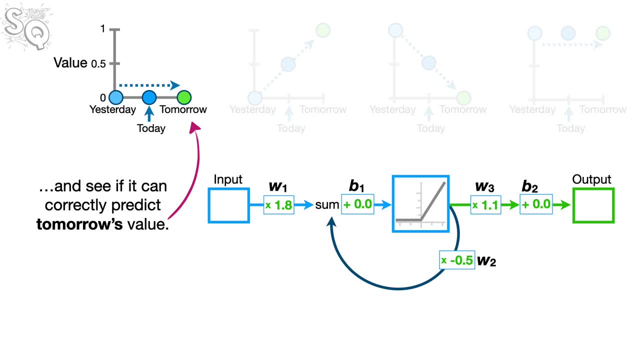 through this Recurrent Neural Network and see if it can correctly predict tomorrow's value. Now, because the Recurrent Neural Network has a feedback loop, we can enter yesterday and today's values into the input sequentially. We'll start by plugging yesterday's value into the input. 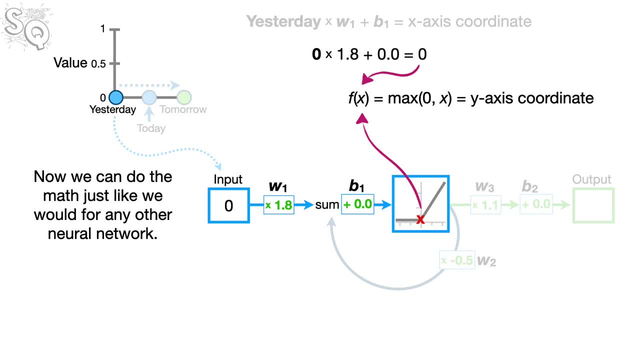 Now we can do the math just like we would for any other neural network. At this point, the output from the activation function- the y-axis coordinate that we'll call y1, can go two places. First, y1 can go towards the output, And if we go that way and do the math, 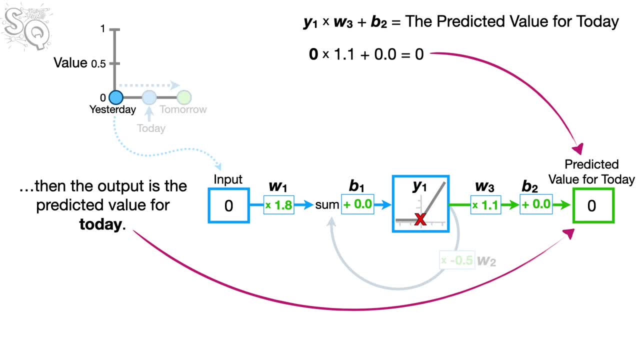 then the output is the predicted value for today. However, we're not interested in the predicted value for today, Because we already have the actual value for today. Instead, we want to use both yesterday and today's value to predict tomorrow's value. So, for now, we'll ignore this output and instead focus on what happens with this feedback loop. 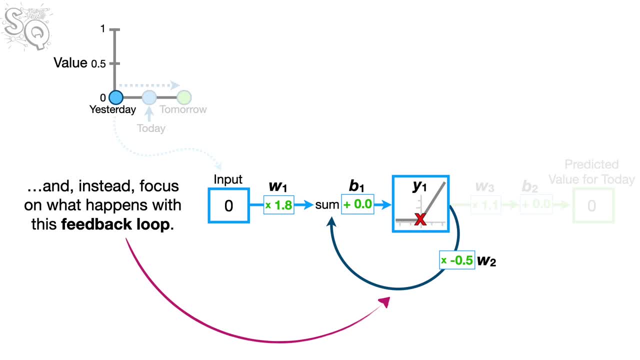 The key to understanding how the feedback loop works is this summation. The summation allows us to infer the value of the value of the new data and when the value included in the jump wave is đâu. The key to understanding how the feedback loop works is this summation. 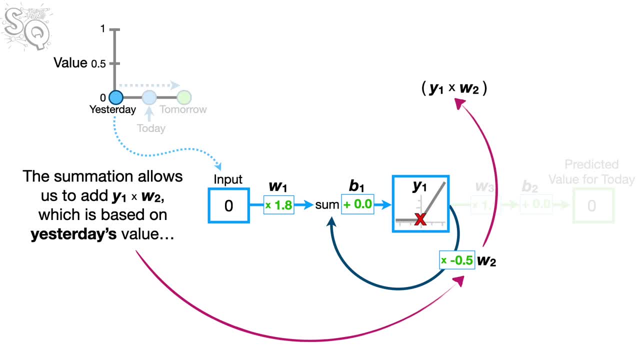 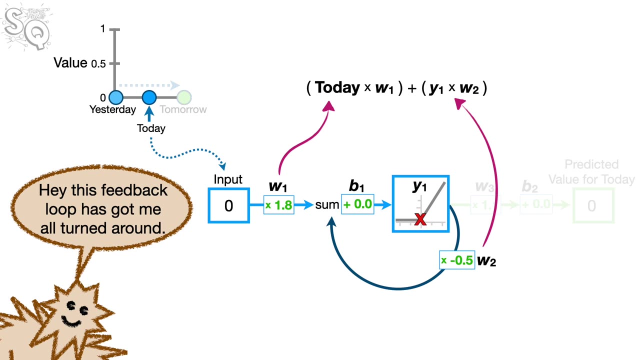 allows us to add y sub 1 times w sub 2,, which is based on yesterday's value, to the value from today times w sub 1.. In other words, the feedback loop allows both yesterday and today's values to influence the prediction. Hey, this feedback loop has got me all turned around. Is there an easier? 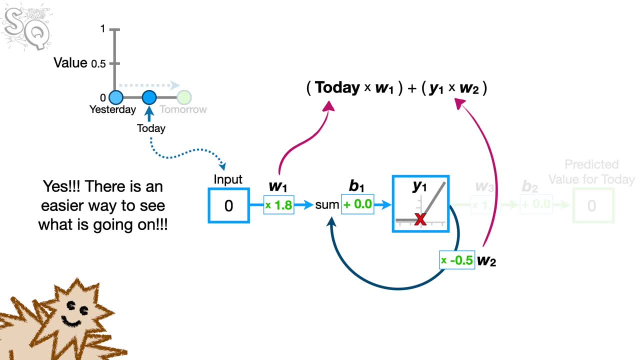 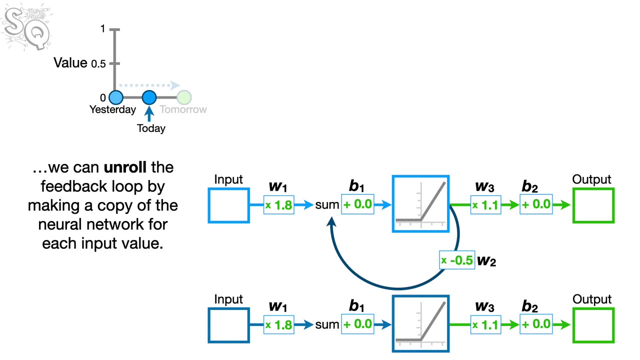 way to see how this works. Yes, there's an easier way to see what's going on. Instead of having to remember which value is in the loop and which value is in the input, we can unroll the feedback loop by making a copy of the neural network for each input value. Now, instead of pointing the 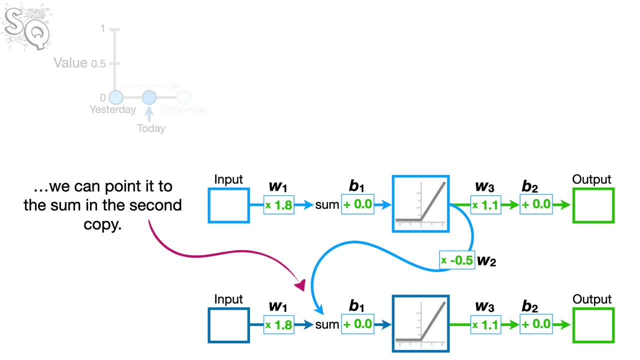 feedback loop to the sum in the first copy. we can point it to the sum in the second copy. By unrolling the recurrent neural network we end up with a new network that has two inputs and two outputs. The first input is for yesterday's. 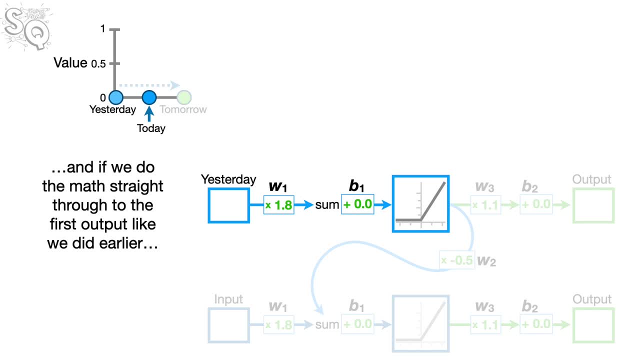 value and if we do the math straight through to the first output, like we did earlier, we get the predicted value for today. However, as we saw earlier, we can ignore this output. The second input is for today's value and the connection between the first activation function. 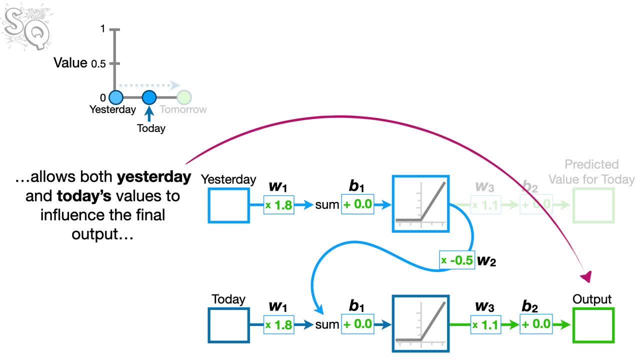 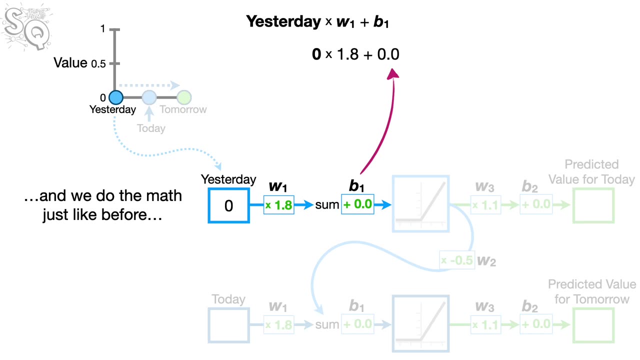 and the second summation allows both yesterday and today's values to influence the final output, which gives us the predicted value for tomorrow. Now, when we put yesterday's value into the first input and we do the math just like before, then we follow the connection from the first. 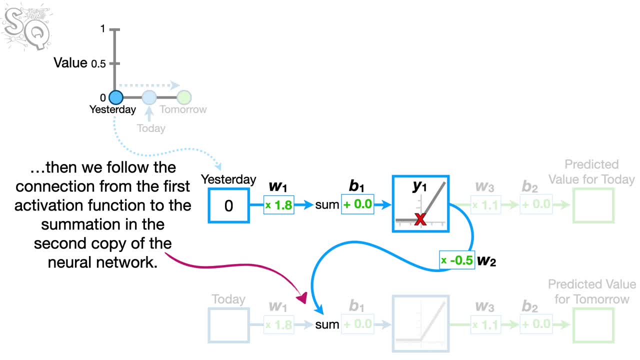 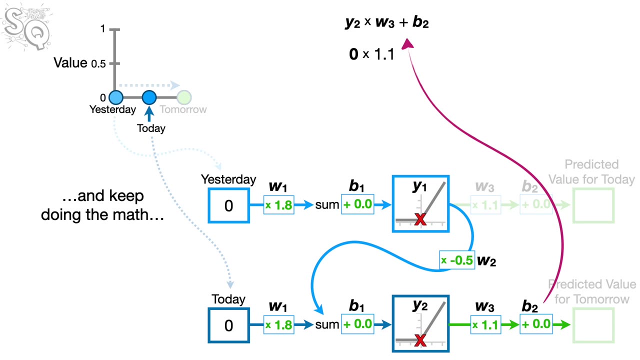 activation function to the summation in the second copy of the neural network. Now we put today's value into the second input And keep doing the math, And that gives us the predicted value for tomorrow, zero, which is consistent with the original observation, In other words, the recurrent neural network correctly predicted. 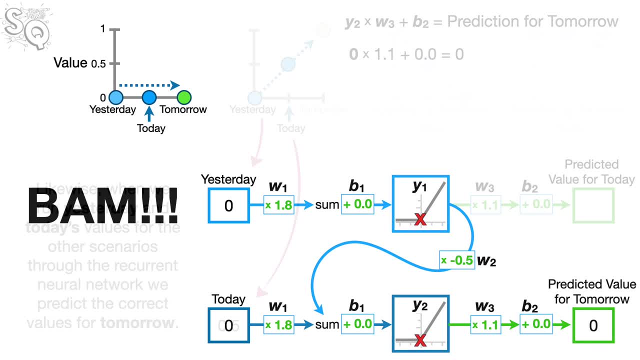 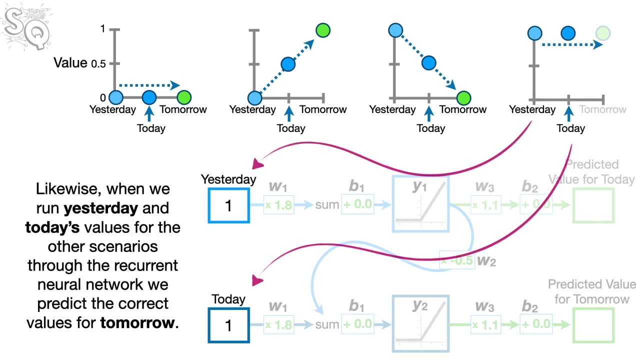 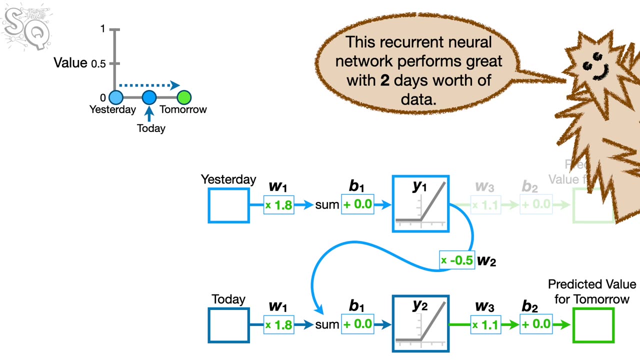 tomorrow's value Bam. Likewise, when we run yesterday and today's values for the other scenarios through the recurrent neural network, we predict the correct values for tomorrow. Double bam. This recurrent neural network performs great with two days worth of data. 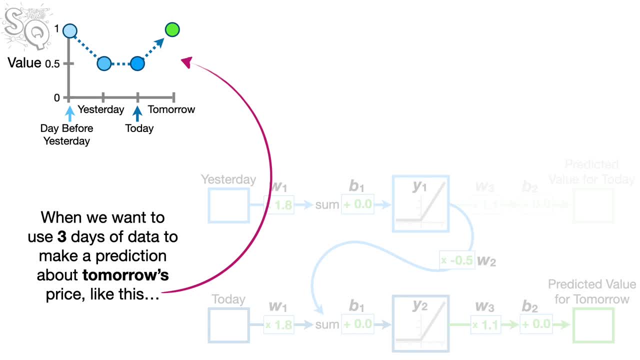 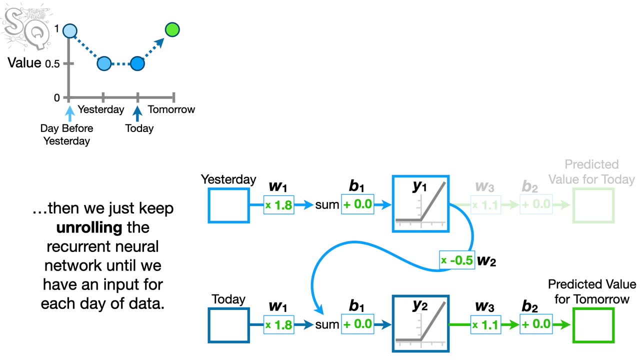 But what if we have three days of data? When we want to use three days of data to make a prediction about tomorrow's price, like this, then we just keep unrolling the recurrent neural network until we have an input for each day of data. 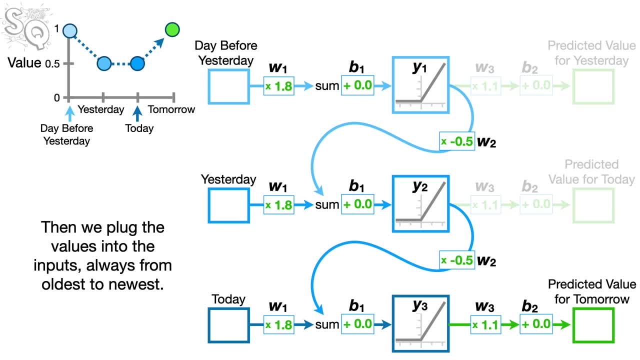 Then we plug the values into the inputs, always from the oldest to the newest. In this case that means we start by plugging in the value for the day before yesterday, Then we plug in yesterday's value and then we plug in today's value. 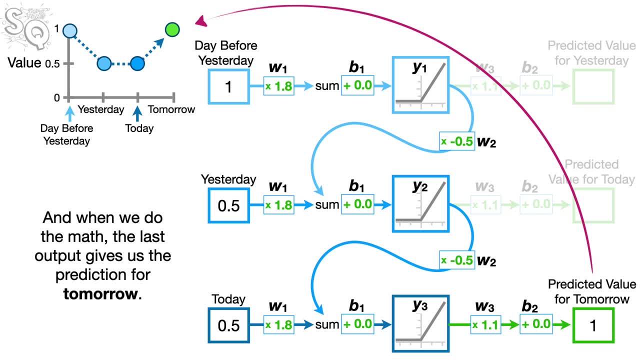 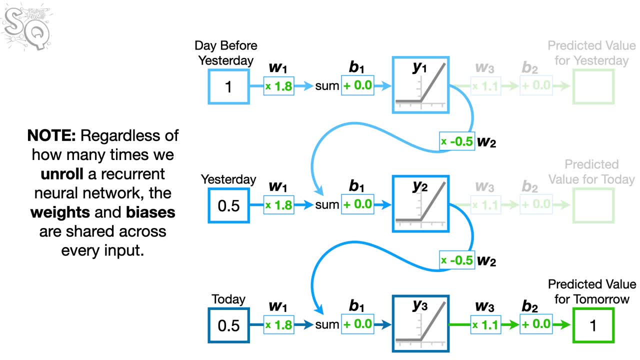 And when we do the math, the last output gives us the prediction for tomorrow. Bam Note: regardless of how many times we unroll a recurrent neural network, the weights and biases are shared across every recurrent neural network. In other words, even though this unrolled network, 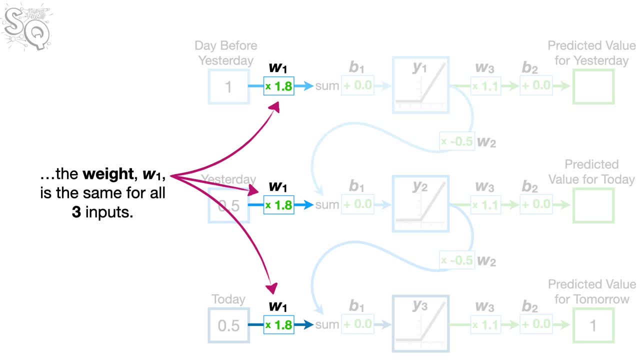 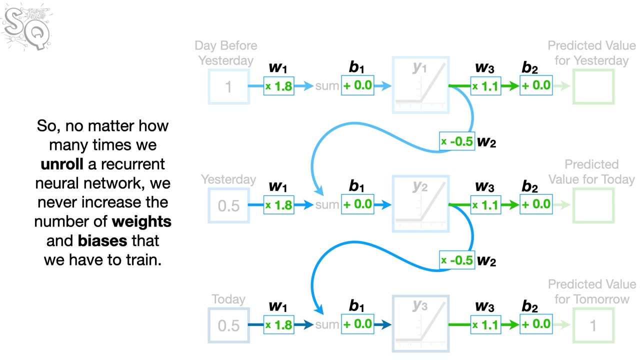 has three inputs. the weight w sub 1, is the same for all three inputs, And the bias b sub 1, is also the same for all three inputs. Likewise, all of the other weights and biases are shared, So no matter how many times we unroll. 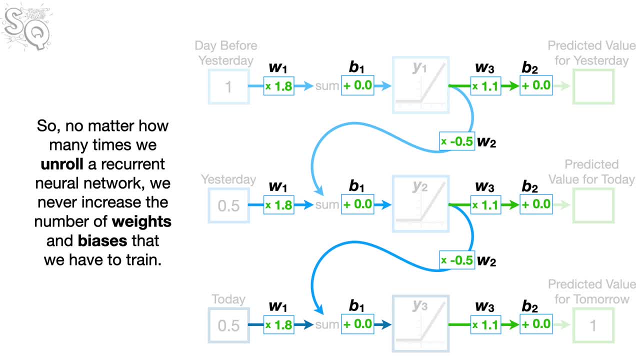 a recurrent neural network, we never increase the number of weights and biases that we have to train Triple bam. OK, now that we've talked about what makes basic recurrent networks so cool, let's briefly talk about why they are not used very often. 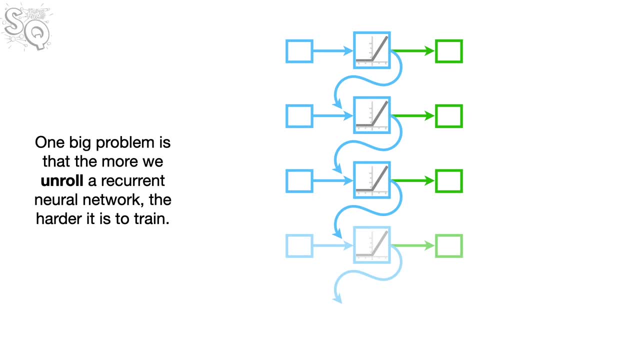 One big problem is that the more we unroll a recurrent neural network, the harder it is to train. This problem is called the vanishing slash exploding gradient problem, which is also known as the hey wait, where did the gradient go? 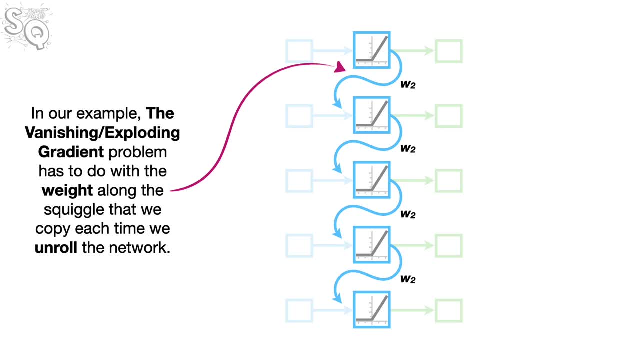 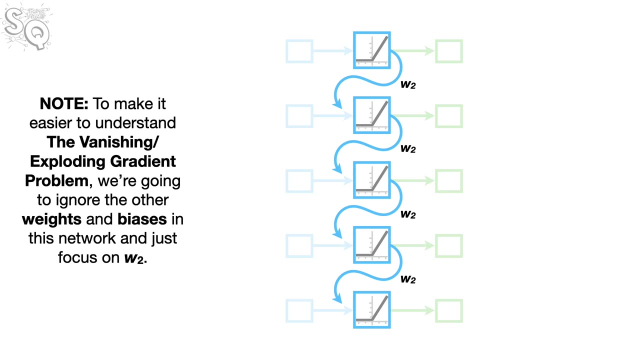 Kaboom Problem. In our example, the vanishing slash exploding gradient problem has to do with the weight along the squiggle that we copy each time we unroll the network. Note to make it easier to understand the vanishing slash exploding gradient problem we're. 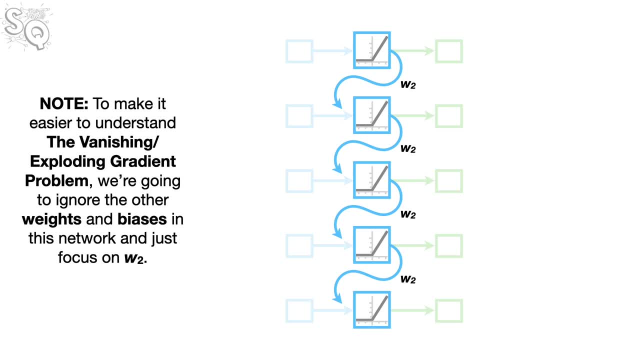 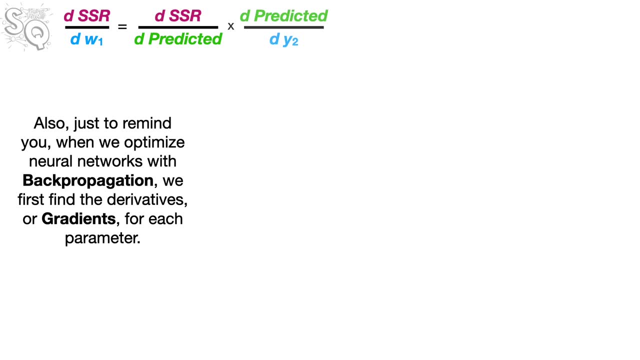 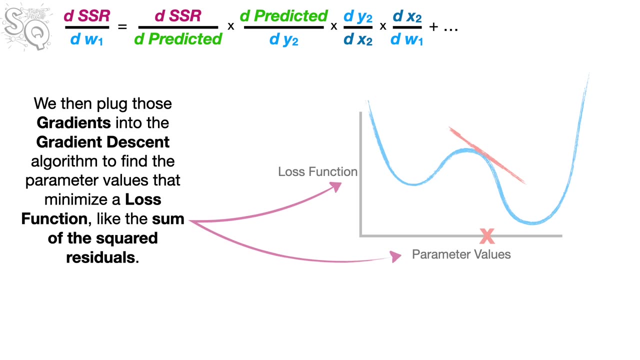 going to ignore the other weights and biases in this network and just focus on w, sub 2.. Also, just to remind you, when we optimize neural networks with backpropagation, we first find the derivatives or gradients for each parameter. We then plug those gradients into the gradient descent. 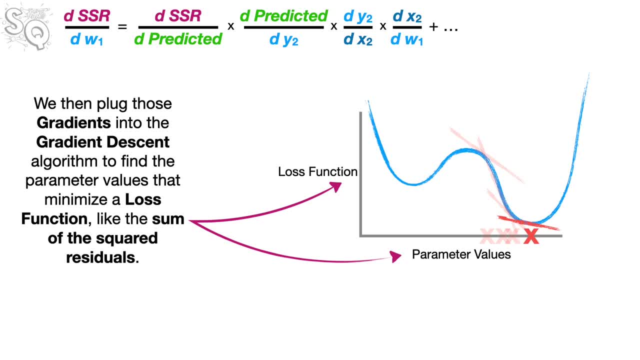 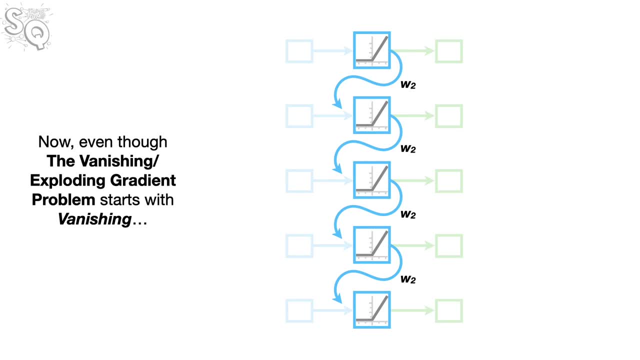 algorithm to find the parameter values that minimize a loss function like the sum of the squared residuals. Bam Now, even though the vanishing slash, exploding gradient problem starts with vanishing, we're going to start by showing how a gradient can explode. 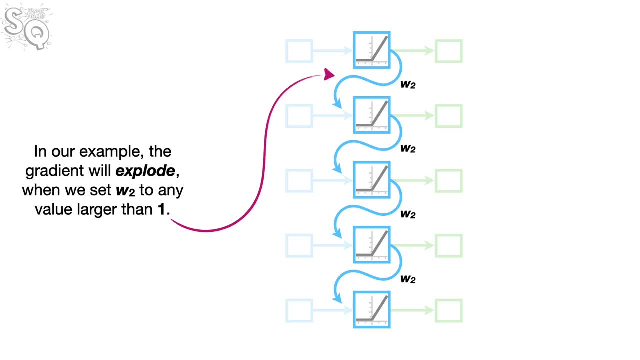 Kaboom. In our example, The gradient will explode when we set w sub 2 to any value larger than 1.. So let's set w sub 2 equal to 2.. Now the first input value: input sub 1,. 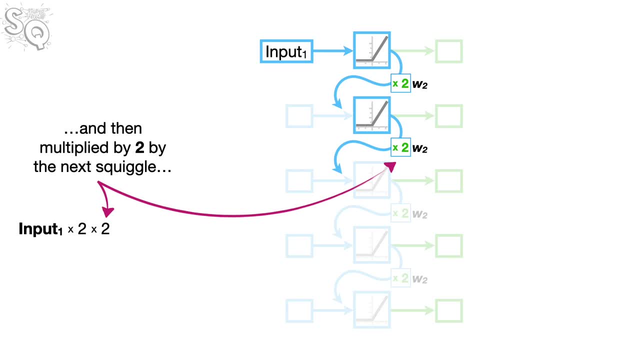 will be multiplied by 2 on the first squiggle, and then multiplied by 2 on the next squiggle, and again on the next squiggle, and again on the last squiggle, In other words, since we unrolled. 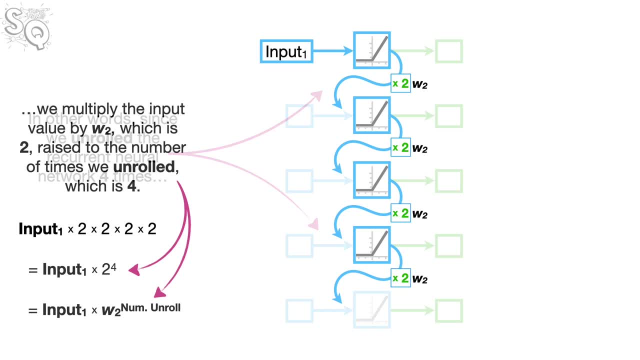 the recurrent neural network four times. we multiply the input value by w sub 2, which is 2, raised to the number of times we unrolled, which is 4.. And that means the first input value is amplified 16 times before it gets to the final copy of the network. 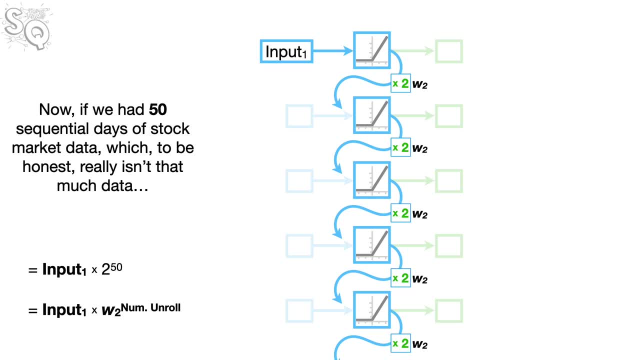 Now, if we had 50 sequential days of stock market data- which, to be honest, really isn't that much data- then we would unroll the network 50 times, and 2 raised to the 50 power is a huge number. 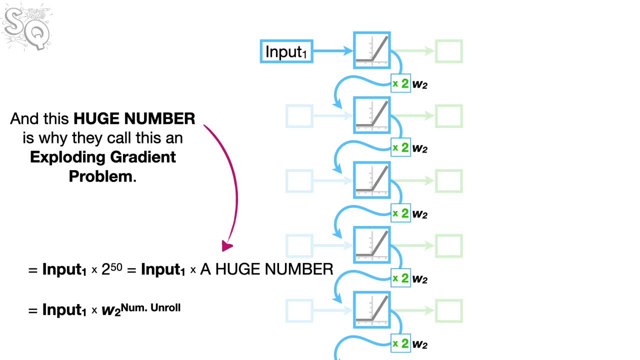 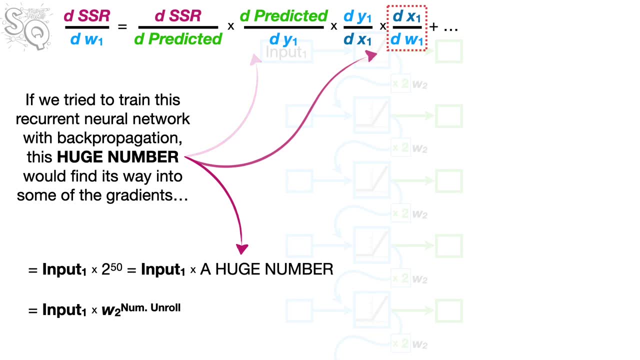 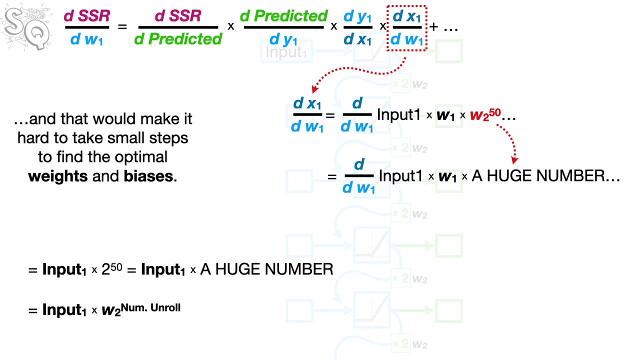 And this huge number is why they call this an exploding gradient problem. Kaboom, If we tried to train this recurrent neural network with back propagation, this huge number would find its way into some of the gradients And that would make it hard to take small steps to find. 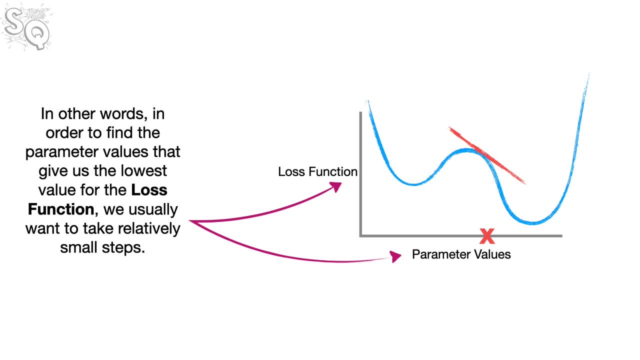 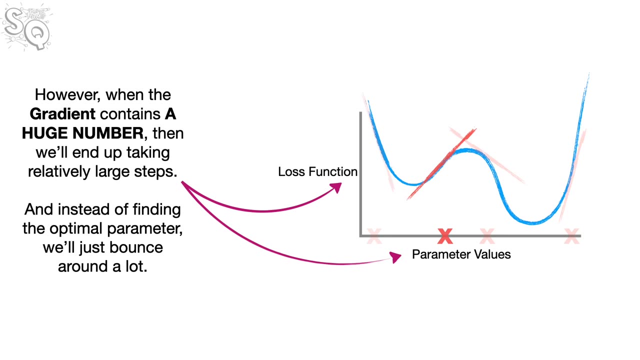 the optimal weights and biases, In other words, in order to find the parameter values that give us the lowest value for the loss function. we usually want to take relatively small steps, Bam. However, when the gradient contains a huge number, then we'll end up taking relatively large steps. 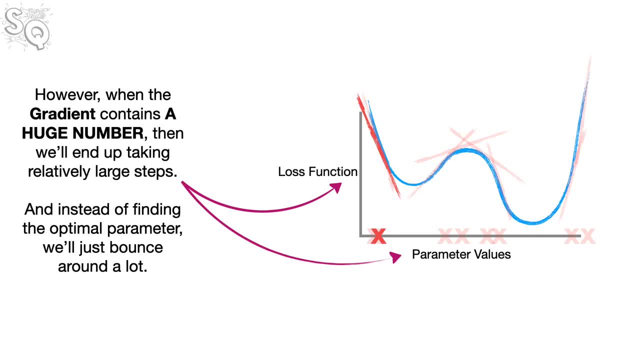 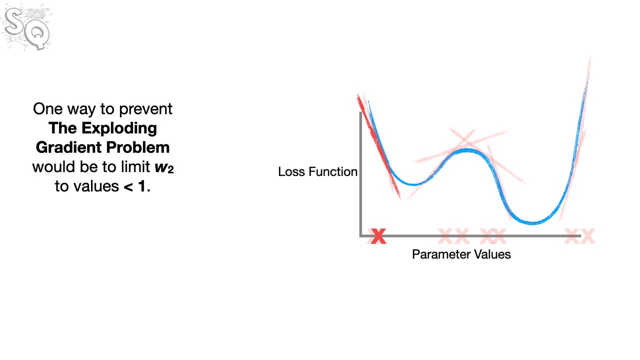 And instead of finding the optimal parameter, we'll just bounce around a lot Wah wah. One way to prevent the exploding gradient problem would be to limit w sub 2 to values less than 1.. However, This results in the vanishing gradient problem. 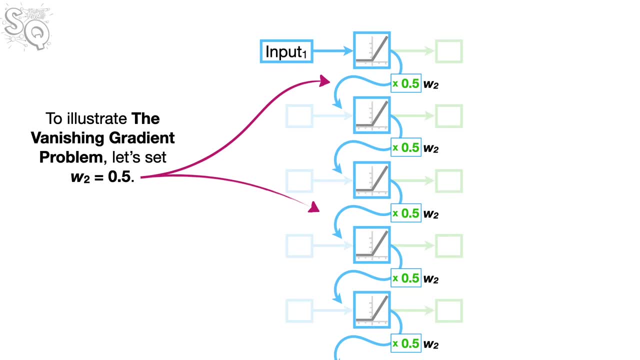 Hey, wait, where'd the gradient go? To illustrate the vanishing gradient problem, let's set w sub 2 to 0.5.. Now, just like before, we multiply the first input by w sub 2 raised to the number of times. 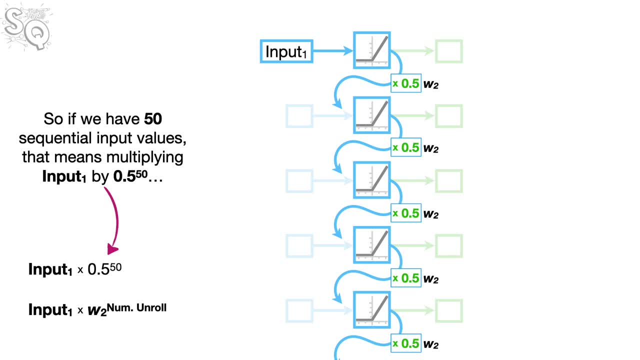 we unroll the network. So if we have 50 sequential input values, that means multiplying input sub 1 by 0.5 raised to the 50th power, And 0.5 raised to the 50th power is a number super close to 0.. 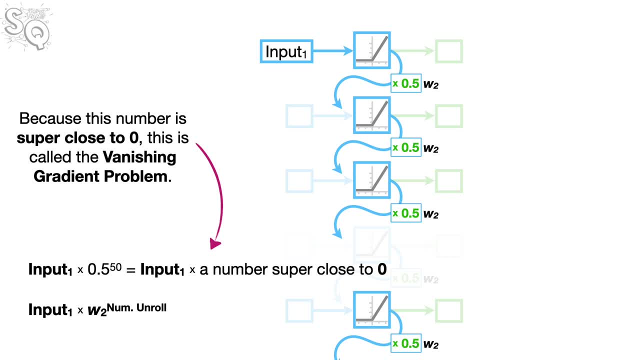 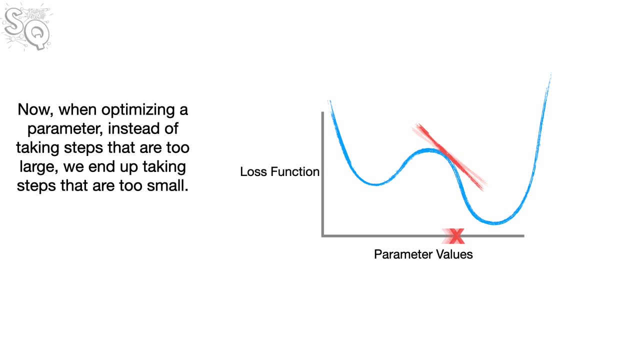 Because this number is super close to 0, this is called the vanishing gradient problem. Now, when optimizing a parameter, instead of taking steps that are too large, we end up taking steps that are too small And, as a result, we end up hitting the maximum number. 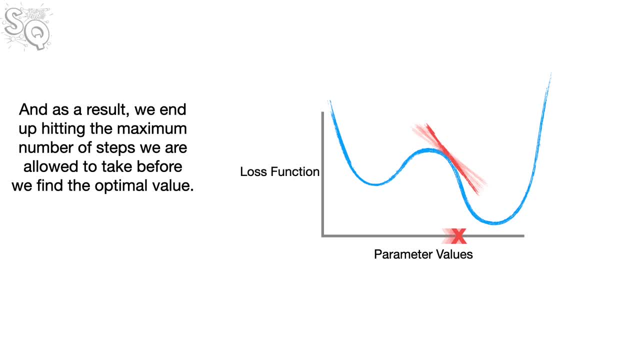 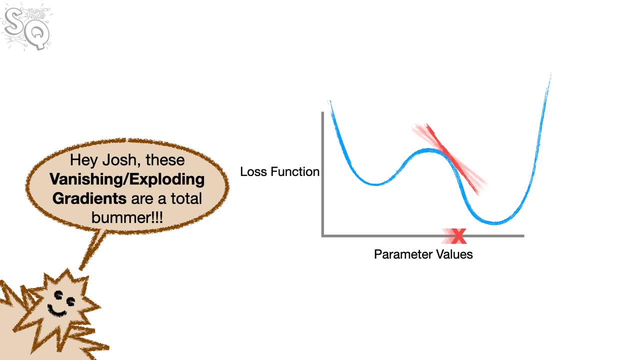 of steps we're allowed to take before we find the optimal value. Wah, wah, Hey Josh. these vanishing slash, exploding gradients are a total bummer. Is there anything we could do about them? Yes, And we'll talk about a popular solution. 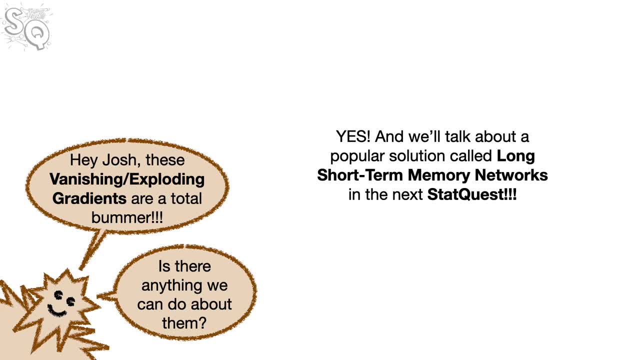 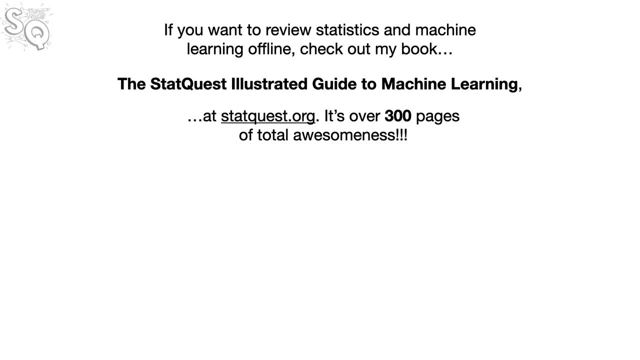 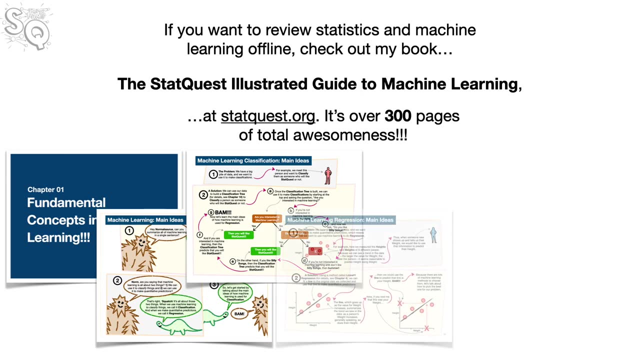 called long short-term memory networks in the next StatQuest Kabam. Now it's time for some shameless self-promotion. If you want to review statistics and machine learning offline, check out my book, The StatQuest Illustrated Guide to Machine Learning.